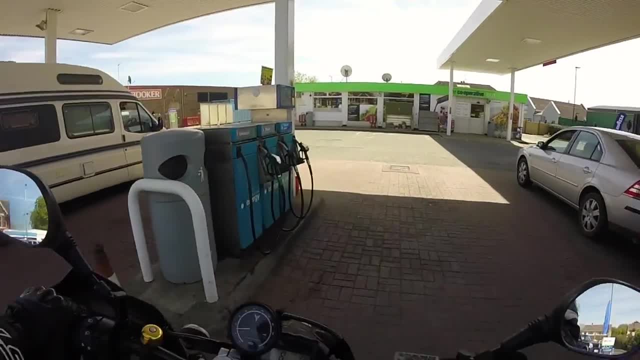 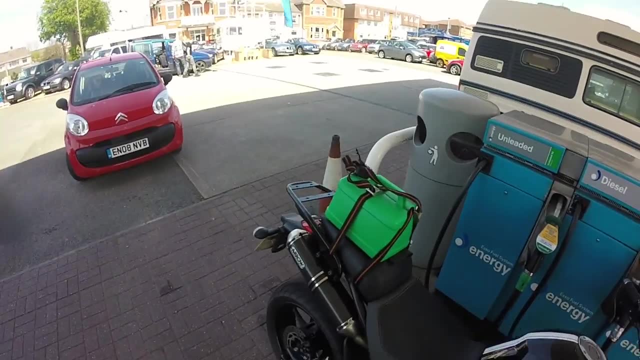 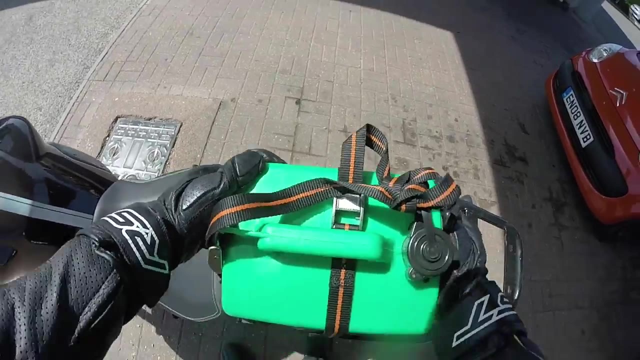 Better not go to the diesel pump. I don't think that will be recommended. I think petrol is more the cool of the day. However, today, I'm not filling that one up. I'm filling that one up, I'll do whatever that is. I ain't going nowhere Knowing the range of your motorcycle. 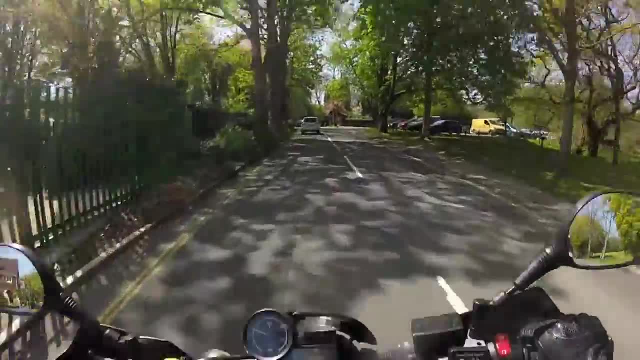 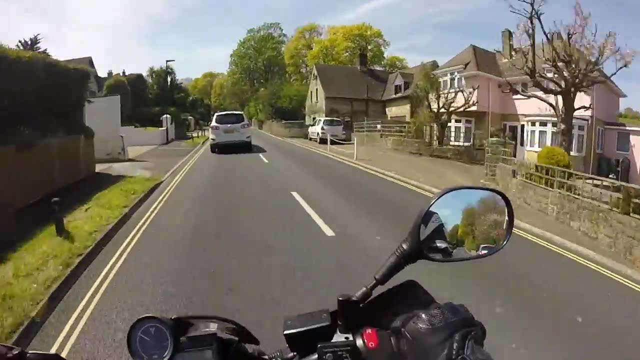 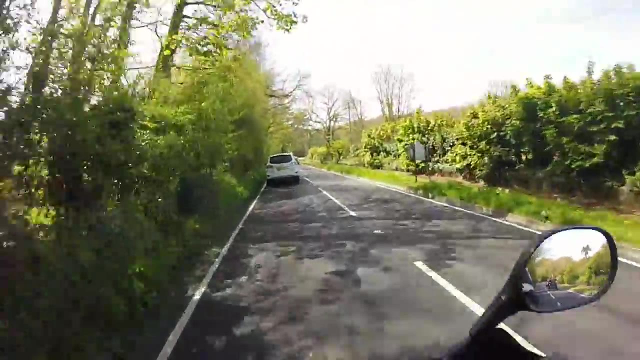 is important because these lights and gauges, they can never be 100% accurate. They're good, they are generally very good, but they can never be trusted 100%. So to know the range, you can calculate. it sort of. once again, not very accurately. 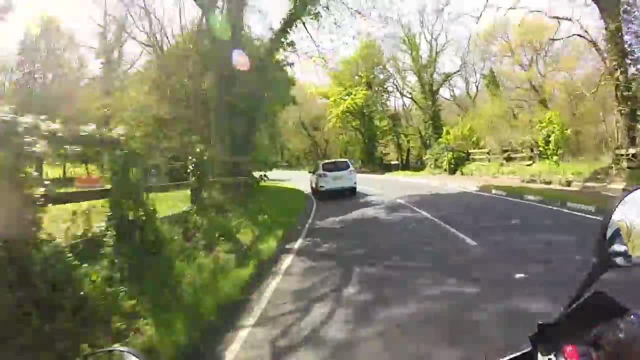 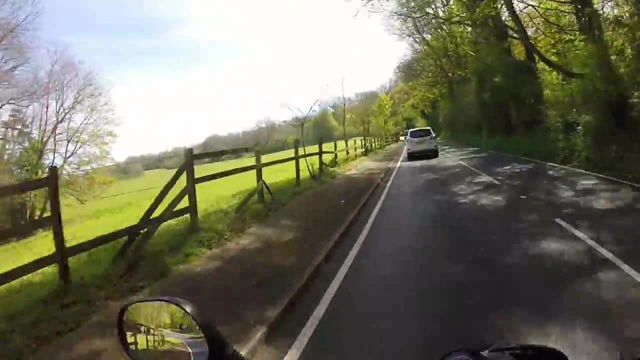 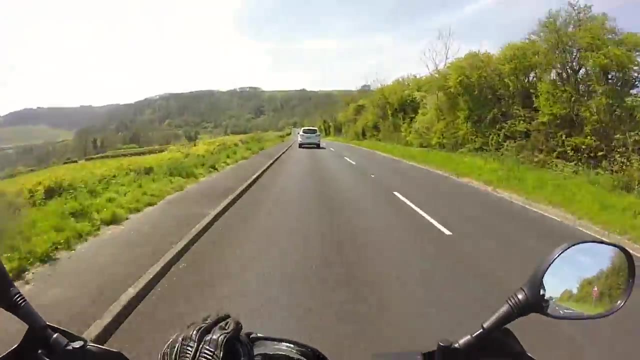 You can calculate the miles to the gallon, then how many litres your tank takes and such like. But then again, the only accurate way of testing it is to actually do it. I always reset my trip when I do filling up. So currently I'm on 133.8 miles. 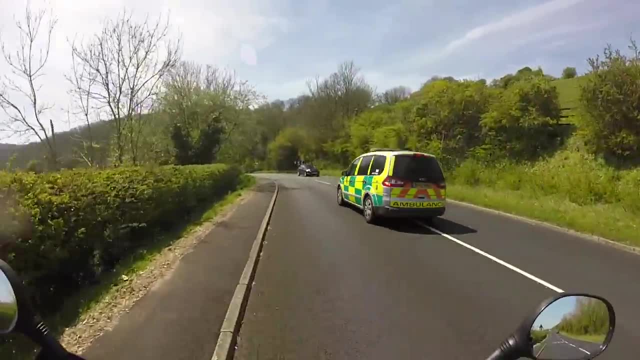 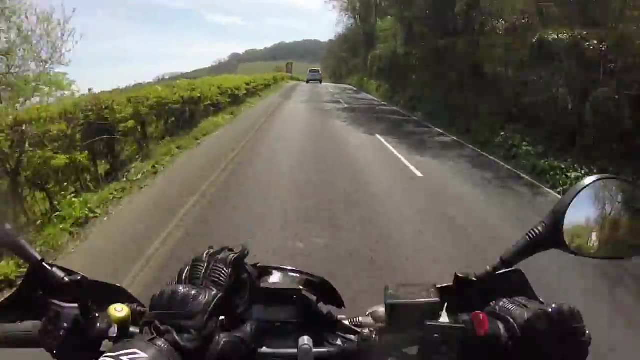 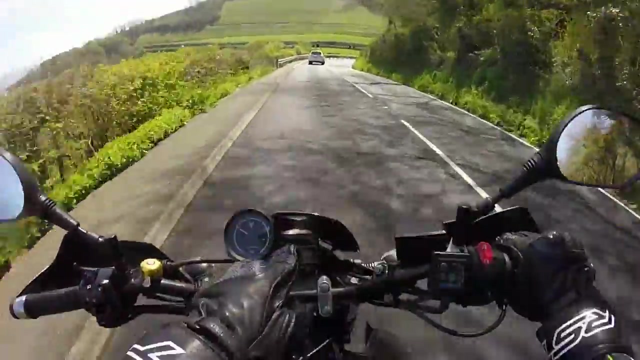 Oh, police in twos behind us. So yeah, 134 miles, there it is, And luckily on the Yamaha MT-03, or they say that it was on the WR as well. When the light does come on, you get a new trip telling you how far. 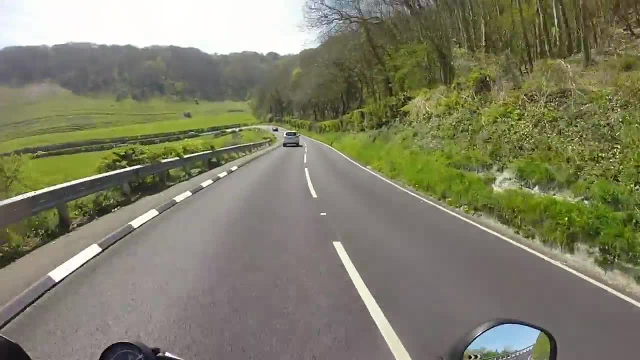 you've gone since the light was active And I've currently gone 17.4 miles, So therefore the light came on at about 115 miles. This is a 15.4 mile. This is a 15.4 mile. 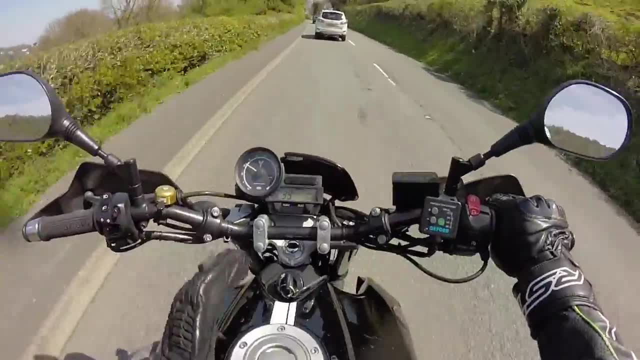 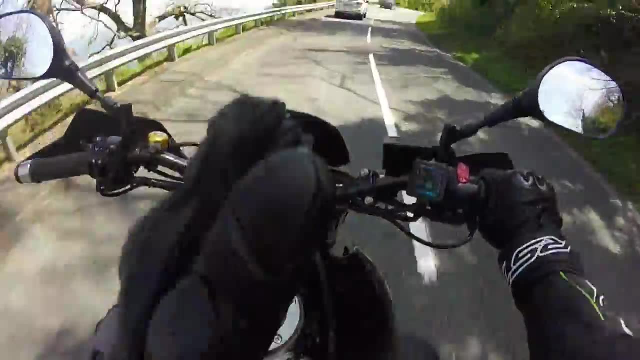 This is a 15.4 mile, a 15 litre petrol tank and the last time I filled it up was on the mainland, on the way back from. Loomies sat on the bike, so it's upright getting as much in there as possible. 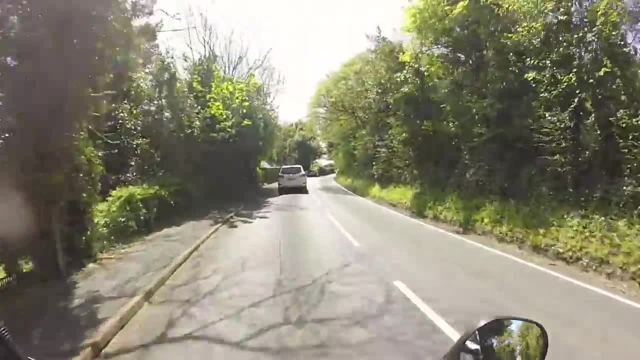 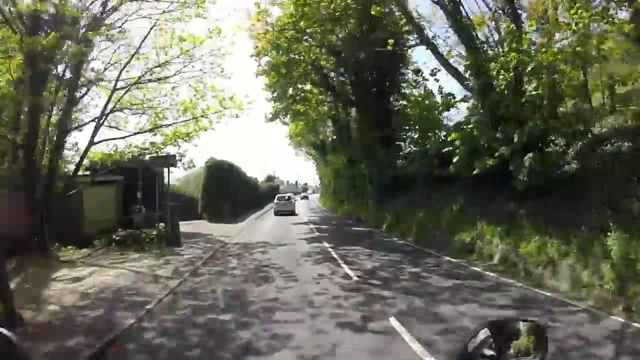 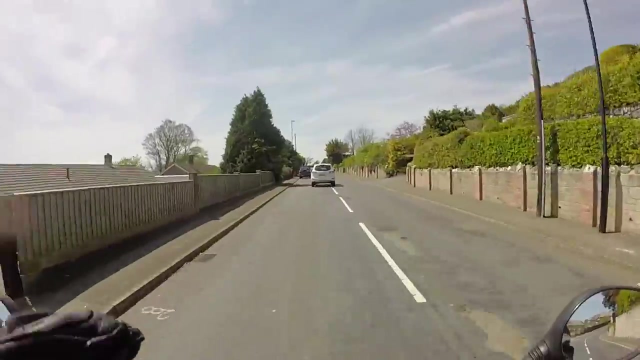 the most amount of fuel in there And according to the Yabaha handbook for this motorcycle, that light comes on when there is four and a half litres of fuel left. So if you do the complicated maths, that would probably get me to about 170 miles or so. Motorcycle News. 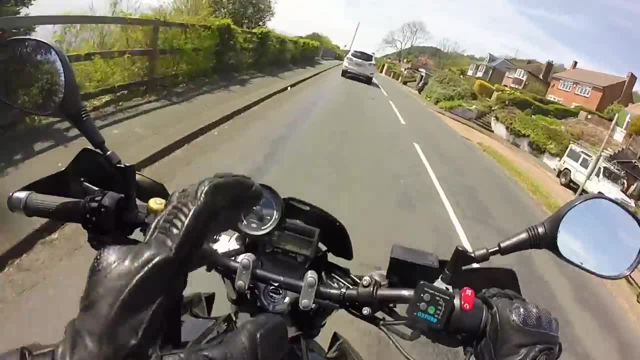 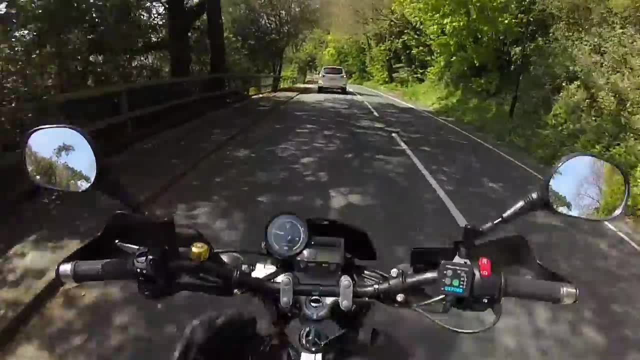 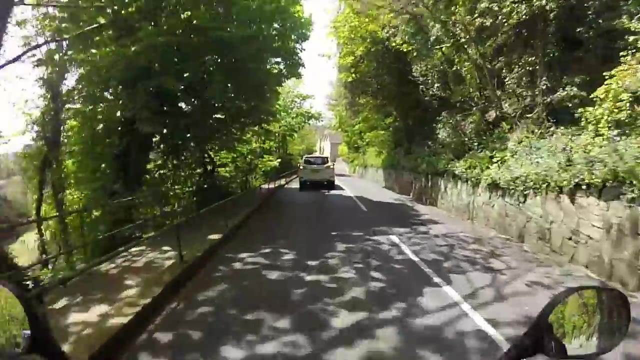 MCN. they reckon 180 on their tests. I think that could be pushing it a bit, But we'll find out. That's the joy of doing this test. I'm not doing anything today, riding wise, that I wouldn't normally be doing, So we'll see how far I get. Place your bets now. I'm. 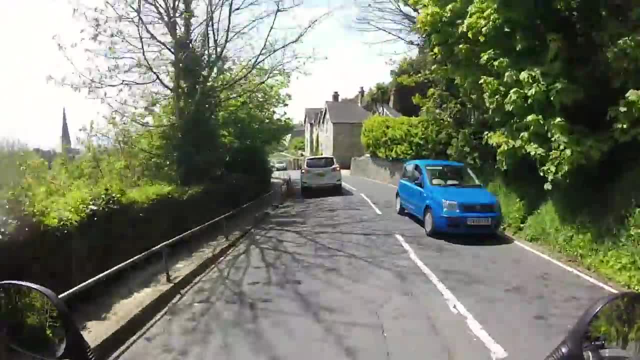 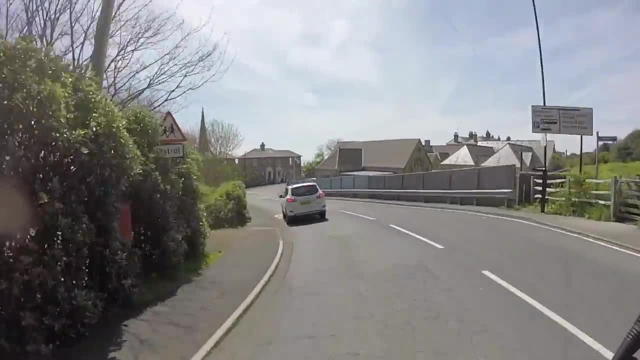 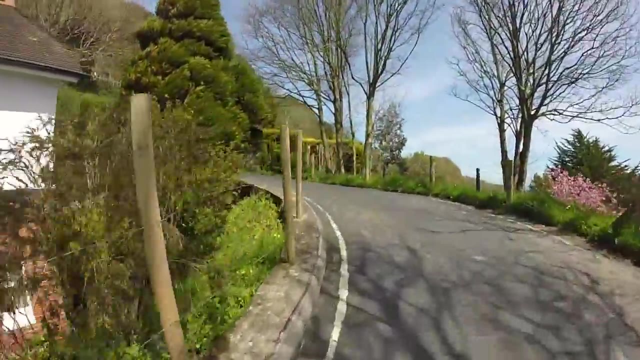 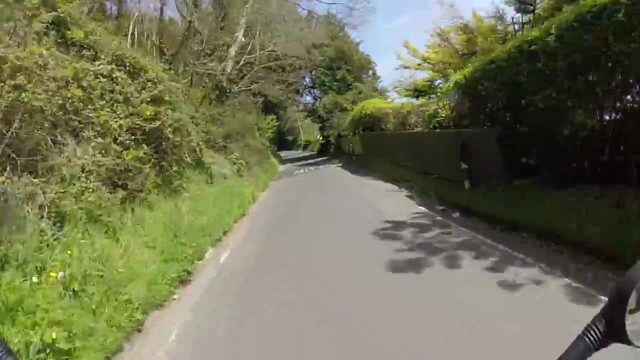 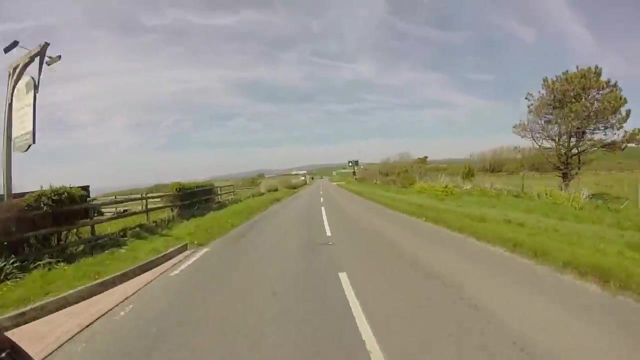 going to say quite simply, a quite simple equation: four and a half litres get me 40 miles, So 45 miles on top of 115 is 160 miles. Don't mind about you, I'm ready for the hill gradient coming up. Look at that. How could I forget High tech? And here we are, the 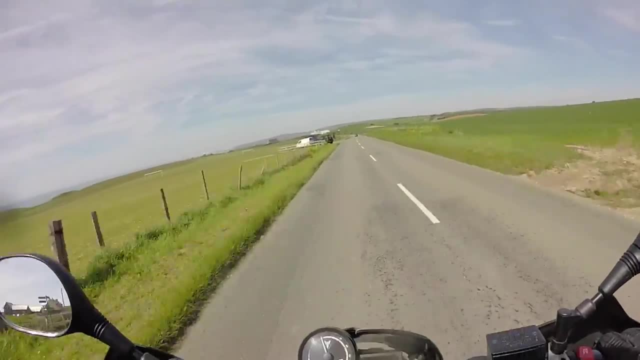 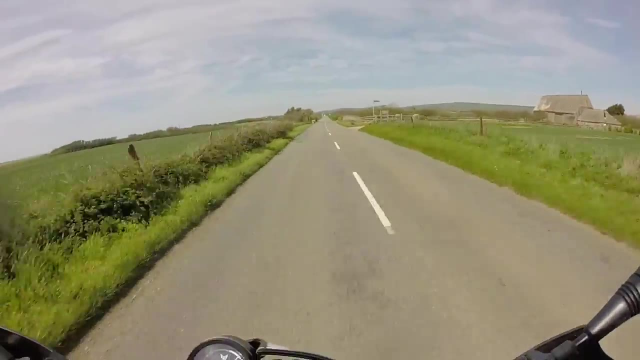 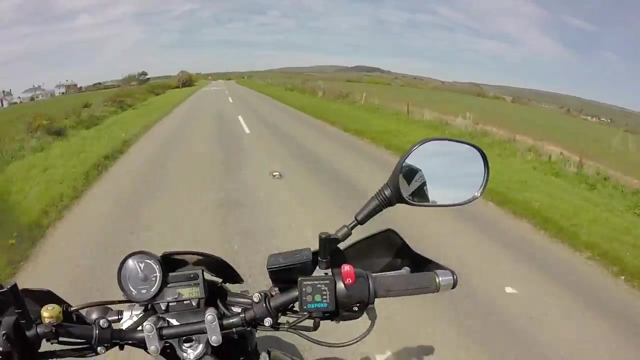 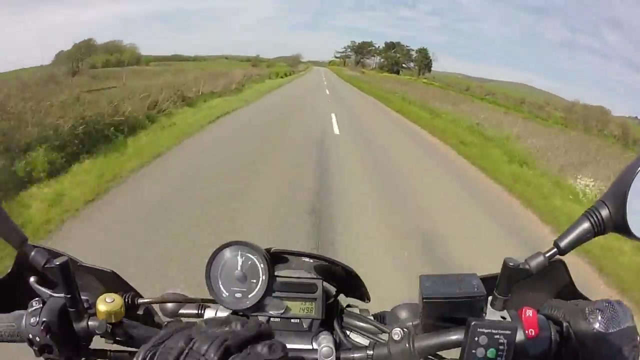 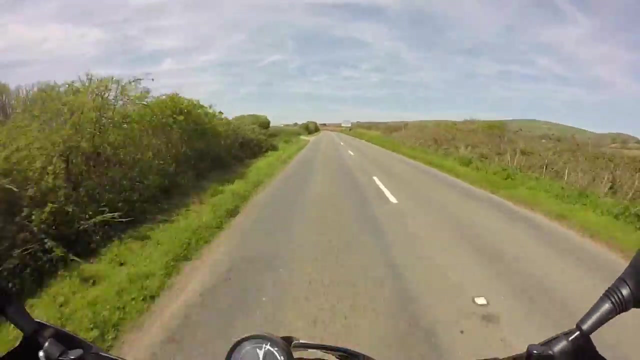 military road Boom. Goodbye petrol buddy. This is so bumpy And calm your tits, And the petrol can is still there, which is a bonus. Yes, we're getting into the unknown now. I haven't gone above 150 miles. We're just about to hit that. There it is 150.2.. 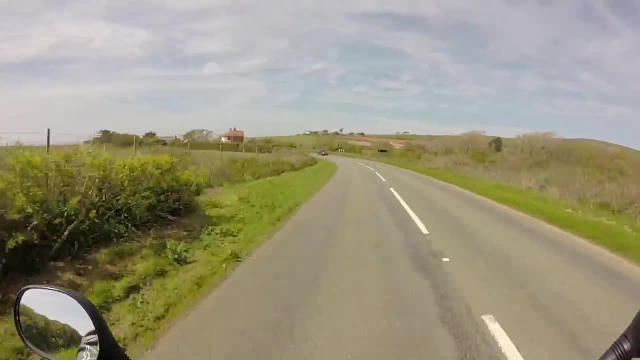 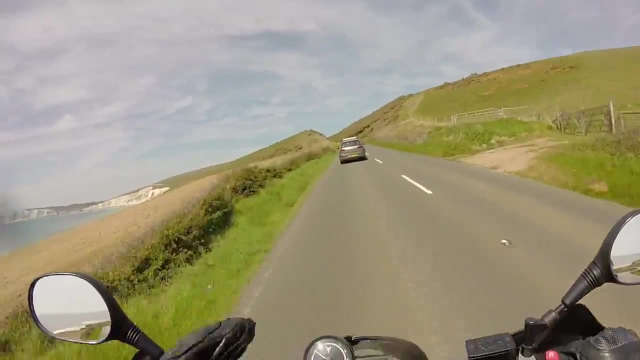 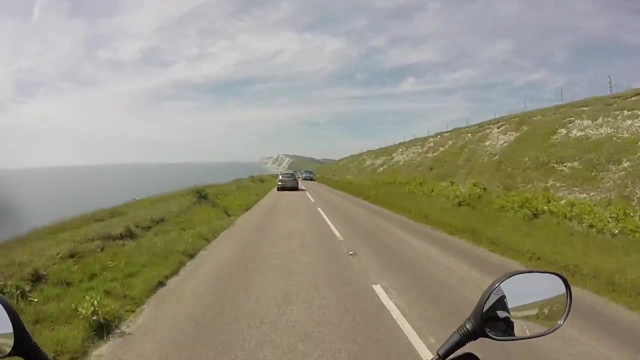 Jesus Miles. This road is ridiculously bumpy. I don't remember it being this bad. More motorcycle tourists. Hey, you can tell they're from abroad. He tilted his head the wrong way. He did the nod the other way around. I think it's possibly possibly the first. 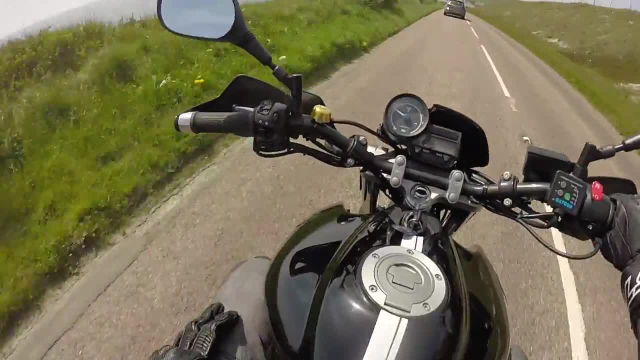 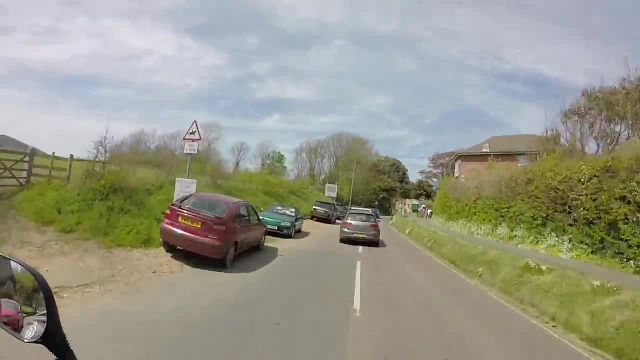 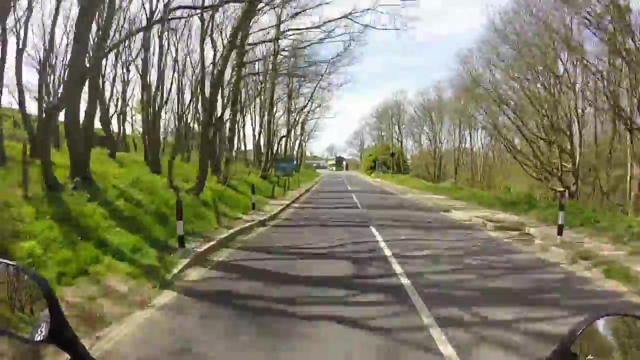 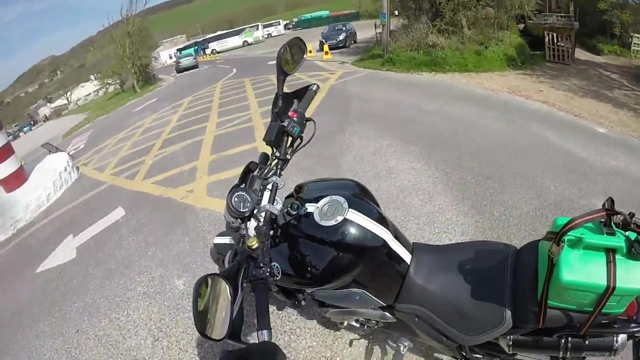 day riding, when I am feeling warmed by the sun- through my trousers I can feel the heat. My prediction of 45 miles is only eight miles away. Welcome to the Needles, Alan Bay. How fantastic. There ain't nothing wrong with that. 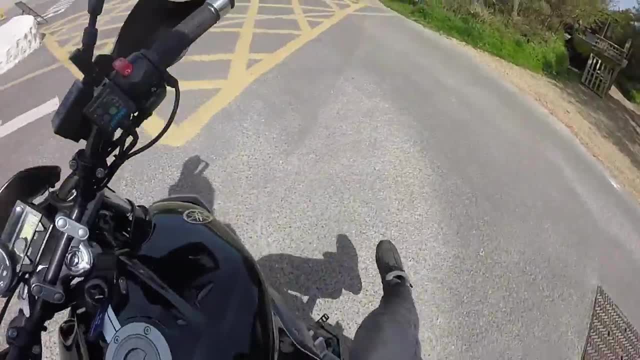 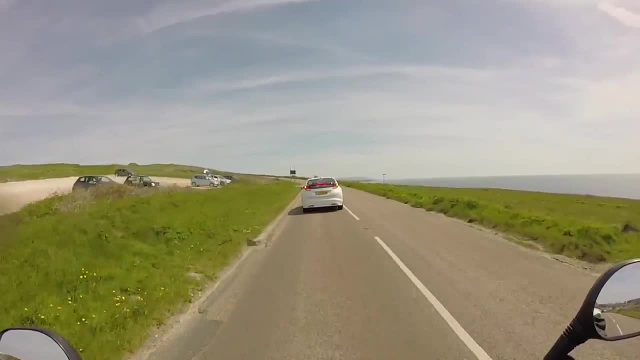 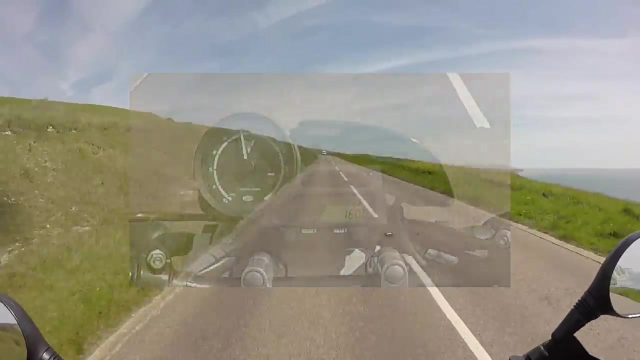 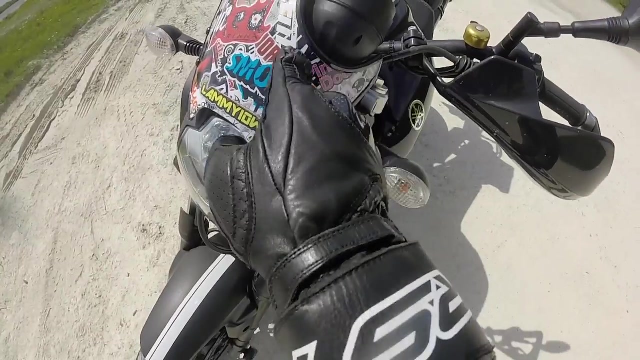 Let's keep going, Wee, Wee. Oh, you're going to the Goat Club darlings. There it is 160 miles now. Seven Four Three, Oh, oh, I've stopped. yes, Pinky doodly sticker is on the screen. 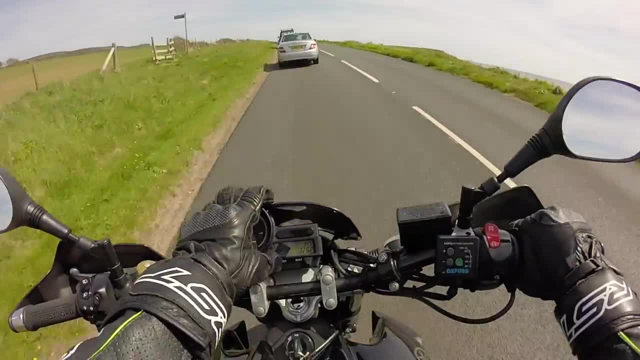 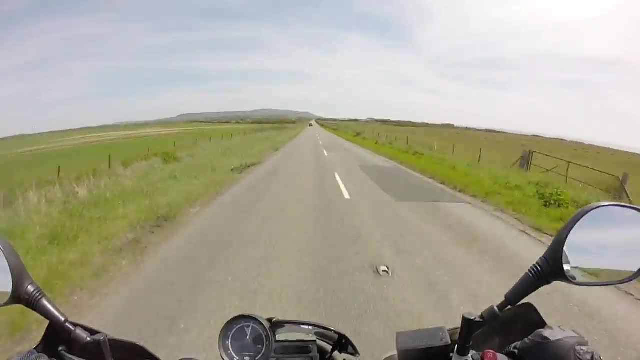 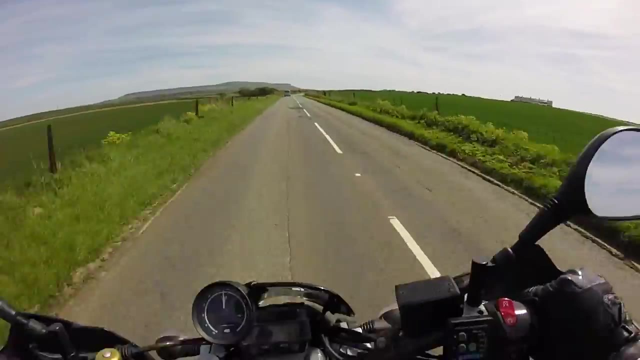 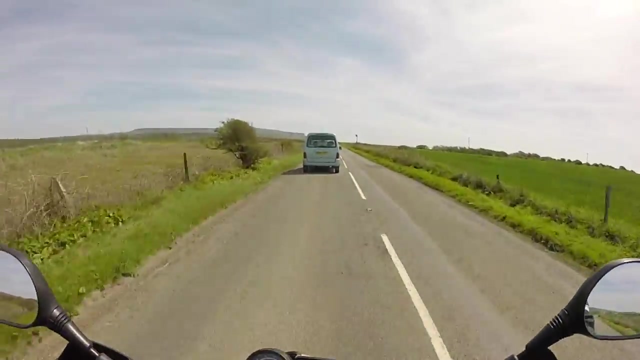 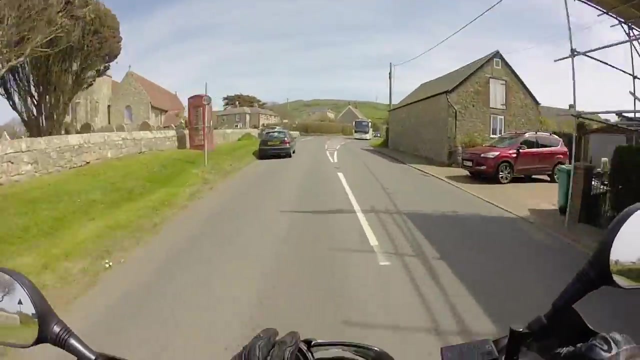 Well, I think there goes my prediction. we have now exceeded 45 miles. The bumps aren't very comfortable coming up to 170 miles. it's got to be a roundabout. now, when it's going to just clonk, That's more than I thought it would go. come on, 170 is about to pop up. 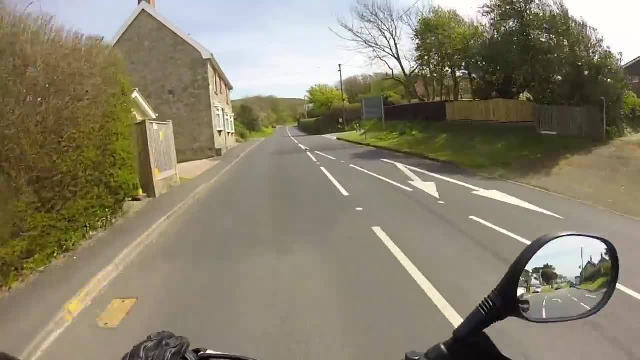 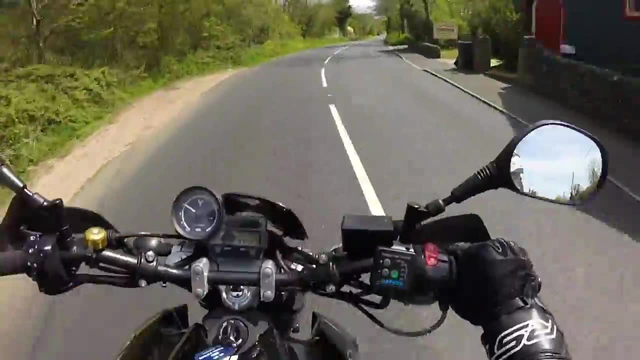 There it is: 170 miles to 15 litres. How much more? How much more is there to go? We've done 53.2 miles since the fuel light came on. There can't be many more miles there, surely? no more than 10 more miles, surely? 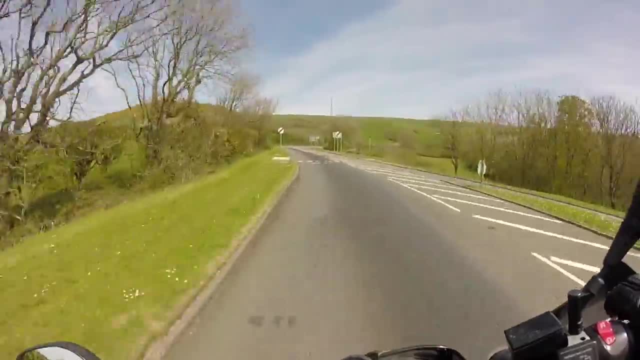 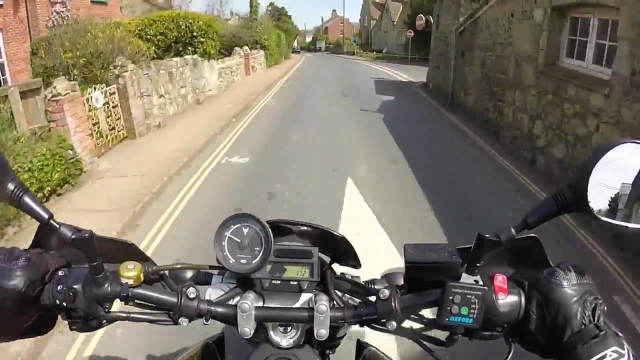 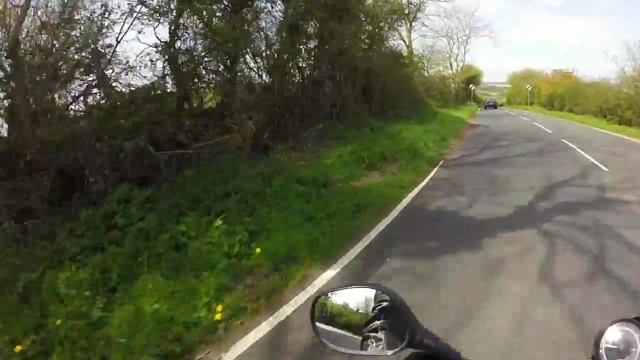 Surely no more than 10 more miles to go. Right, I think we're going to have to go up to Newport, right into the middle of the island. then, On 172.1 miles, let's go to Newport. Whoa pheasant. 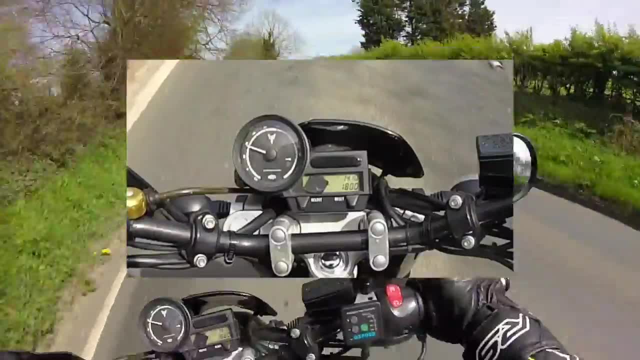 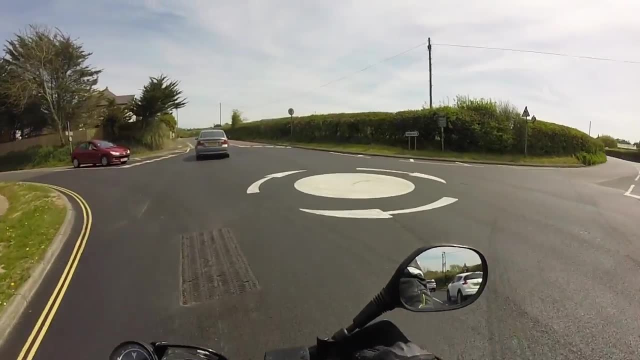 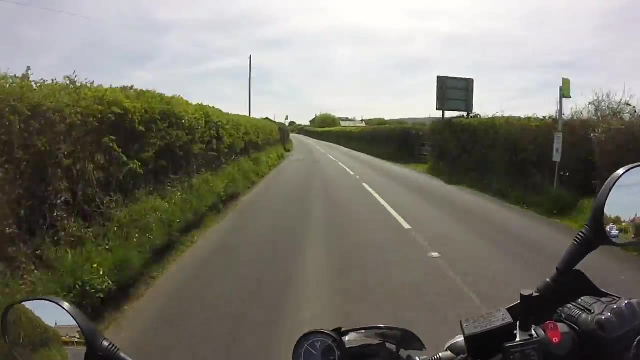 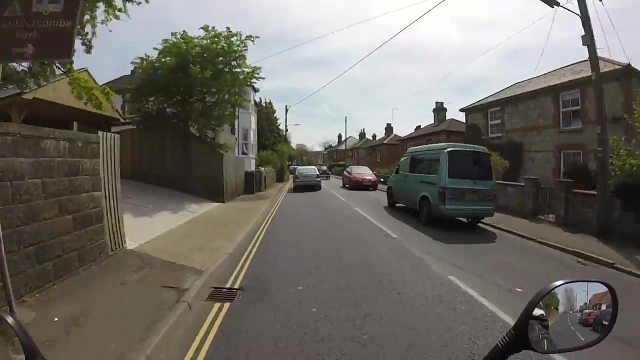 There it is: 180 miles. Oh look, a petrol station Not yet. Surely it can't go much further. Those final four and a half litres are really stretching their legs. Don't want to filter, though, in case I run out of fuel halfway through filtering. 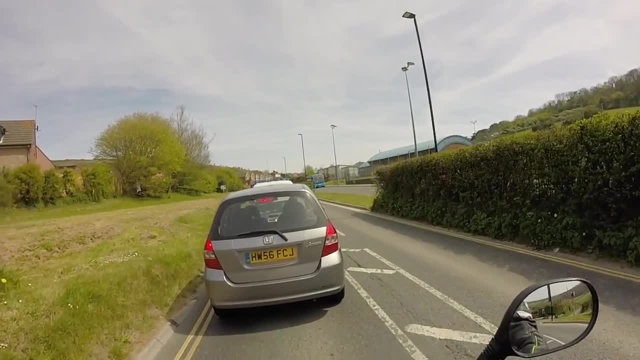 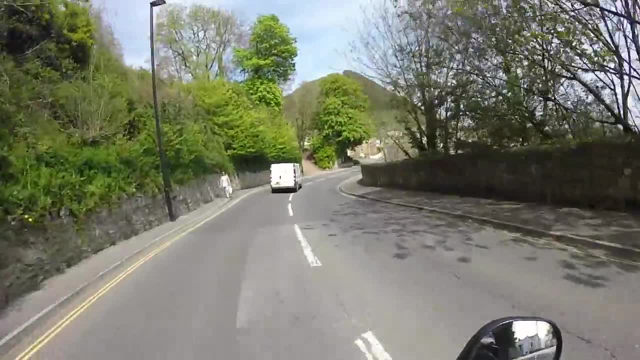 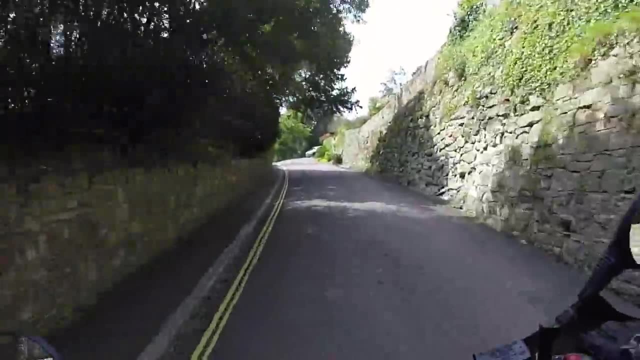 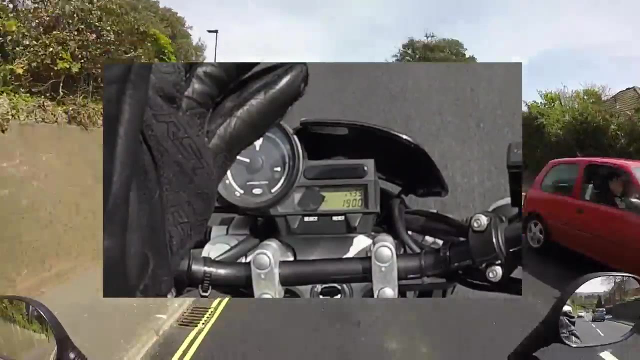 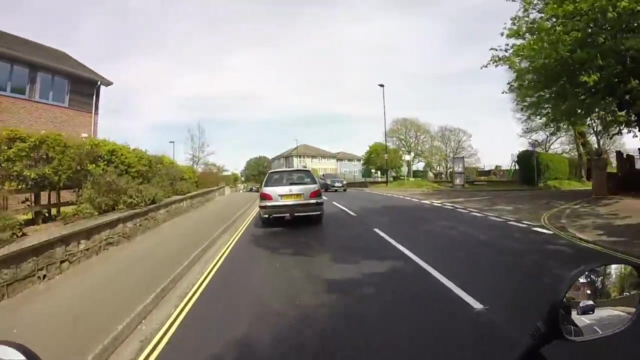 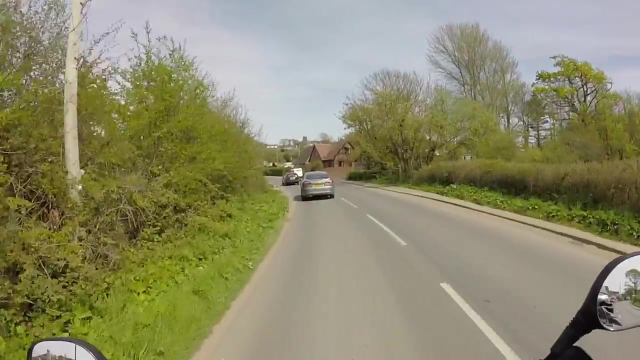 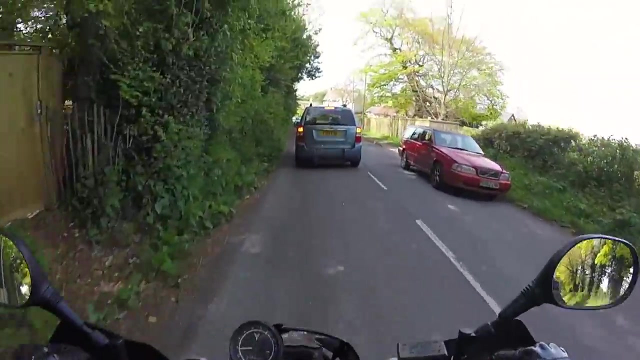 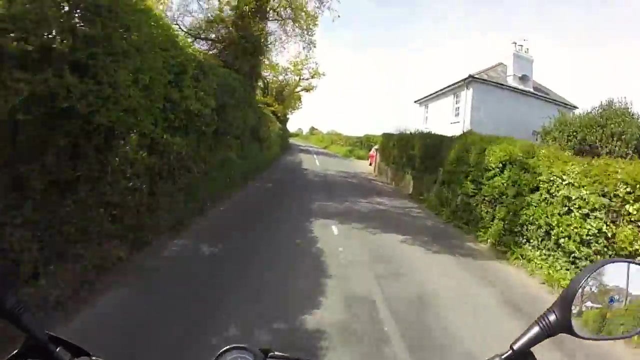 That wouldn't be preferable. Surely 190 is completely out of the window. It has to be There. it is 190 miles. How are you still running? I never thought it would get this far. Nowhere near There. it is 195.. This has got to be the end soon. It cannot get to 200.. I don't believe. 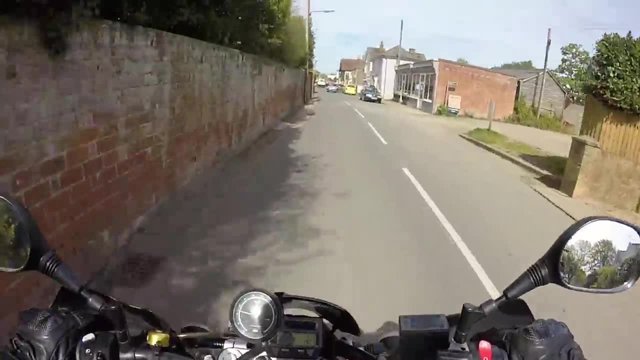 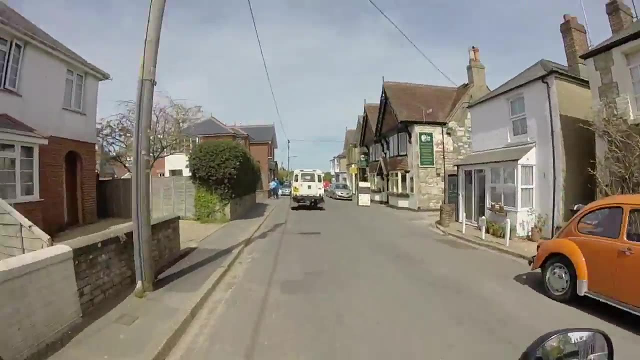 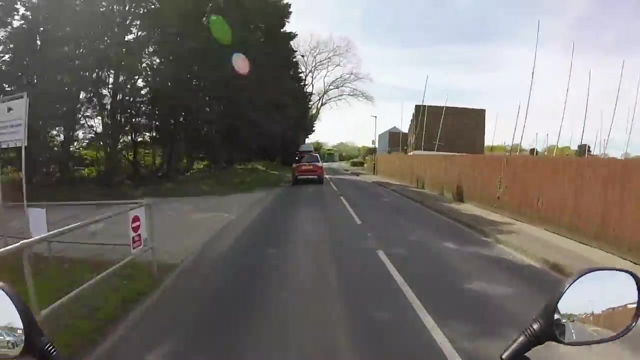 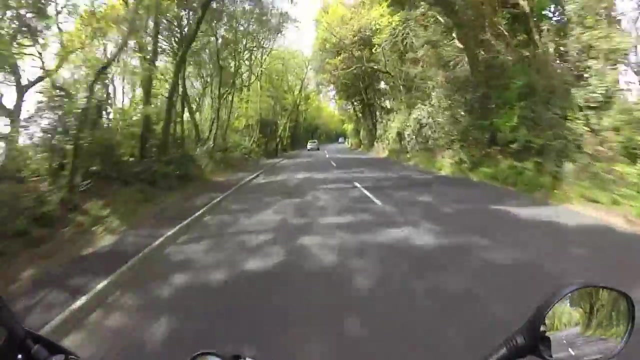 it will. What was my original prediction? 45 when the light came on, so that would have been about 160.. Here we are knocking on the door of 200.. I'm just trying to find a place to go now to get the miles up. 197.. 200, there it is. How much further have you got?